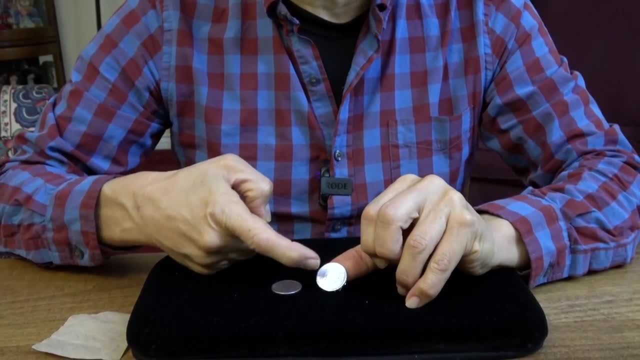 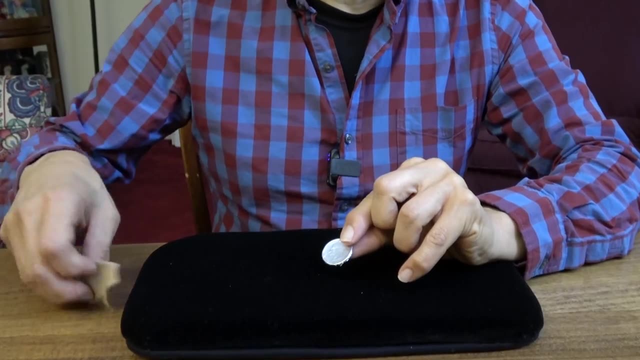 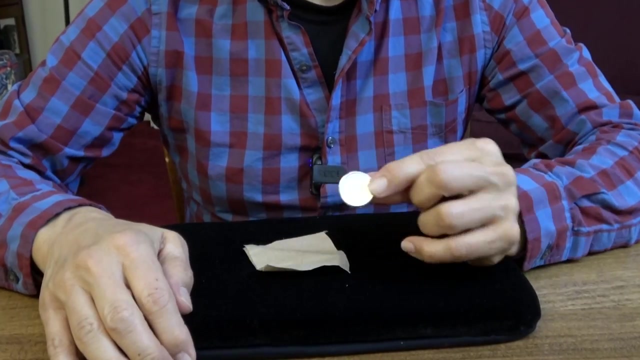 Now, you can't show these side by side And, by the way, I'm using the dull side of the coin. So remove the real coin and you just bring out this coin, You wrap it in a piece of tissue or paper, whatever it is, and you just crumple the whole. 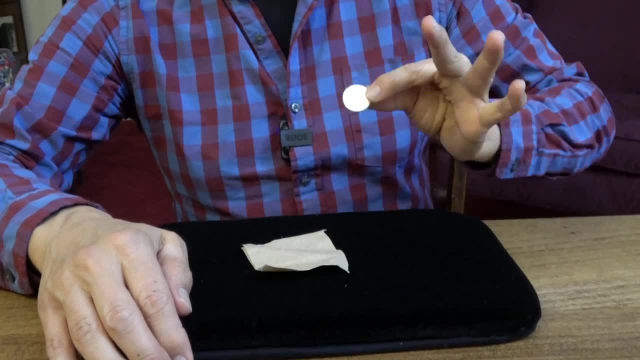 thing up and the coin appears to vanish And you probably want a little distance. You don't want to be showing the coin up close like that. You don't want to be showing the coin up close like that. You don't want to be showing the coin up close like that. You don't want to be showing the coin up close like this. 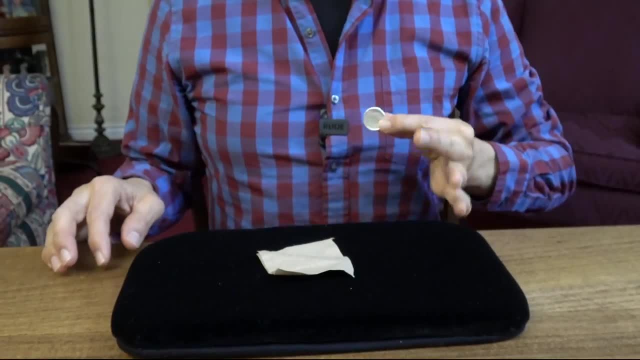 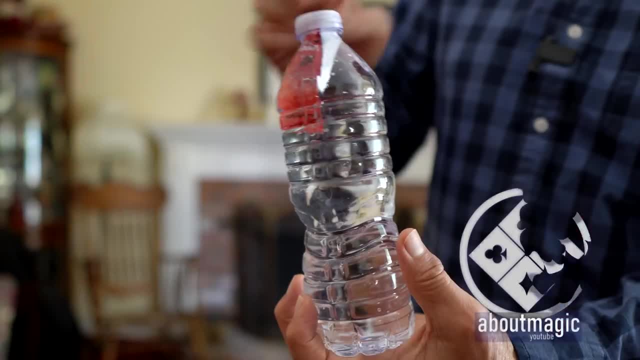 Because then you can pretty much see that it's not a real coin. But if it's back here it looks like a real coin. Now you fill your bottle with water. First of all, you may have to balance the packet that's inside of the water here. 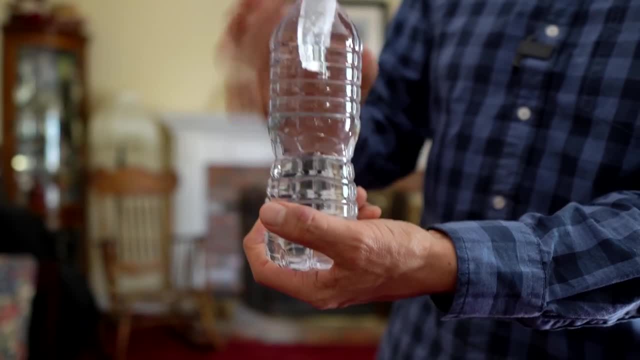 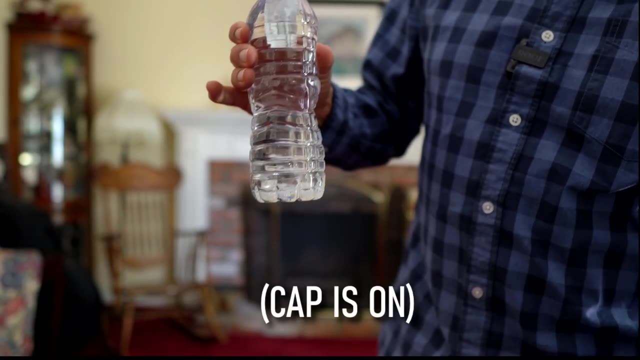 Turns out, I had to use two paper clips, so it was just at that right point. So if it sinks to the bottom, you have too big of a paper clip on it. If it stays at the top and you can squeeze it with the water all the way to the top.